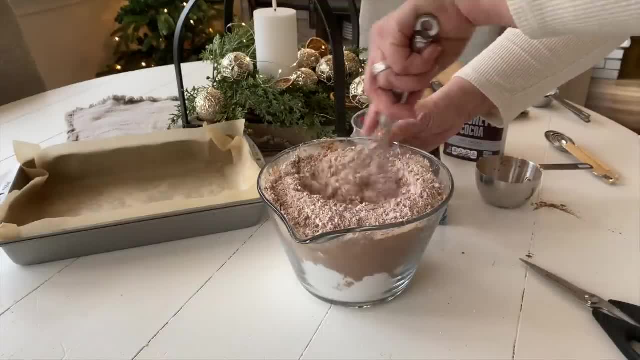 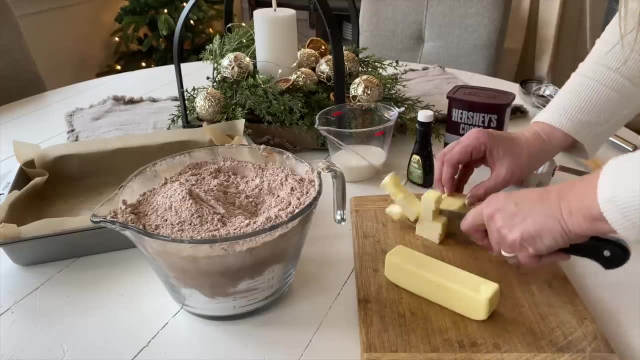 powder. I'm going to mix it together in a microwave safe bowl and then I'm going to cube two sticks of unsalted butter and add that on top of the mixture, along with a half a cup of milk, And I'm not going to mix this together- and then I'm going to microwave this for three to four minutes. 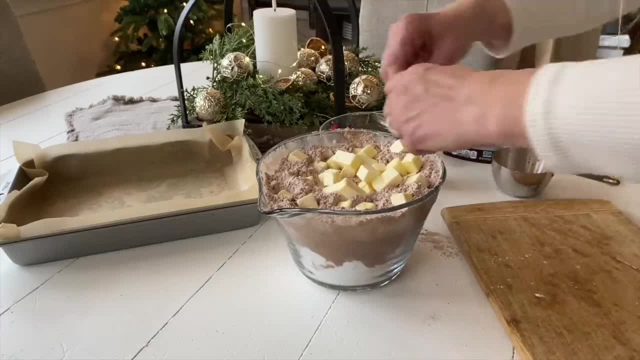 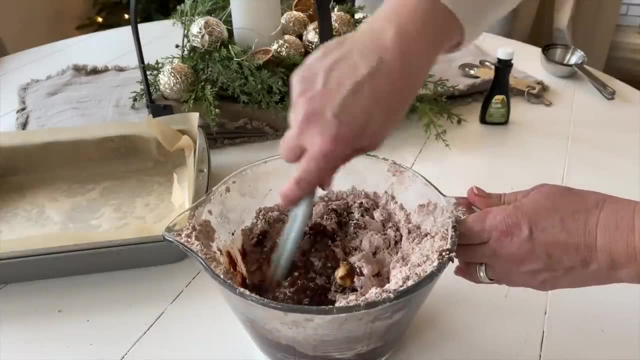 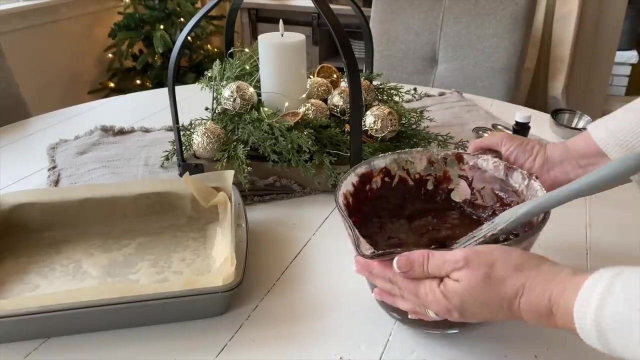 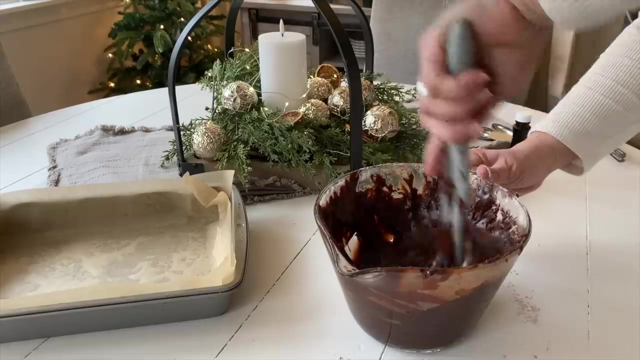 After three minutes, this is how the mixture looks, So I'm going to give it a good stir and then pop it in the microwave for another minute. After four minutes, this is how the mixture looks. It's nice and creamy. Now I'm going to stir in a few tablespoons of vanilla extract. 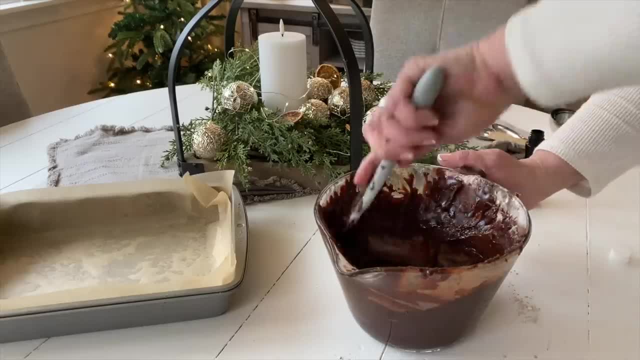 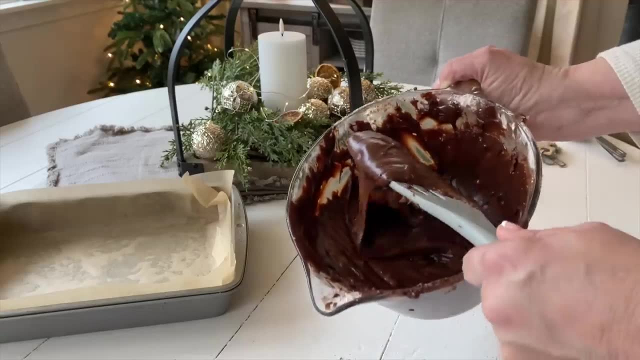 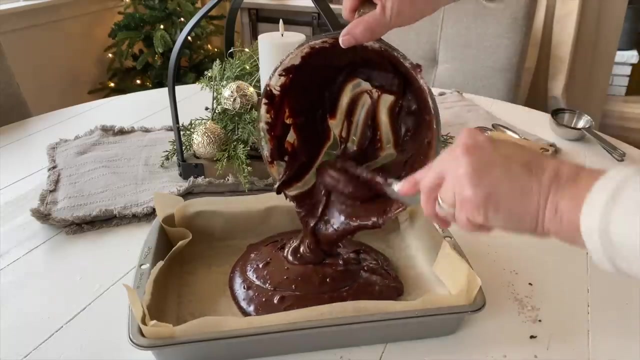 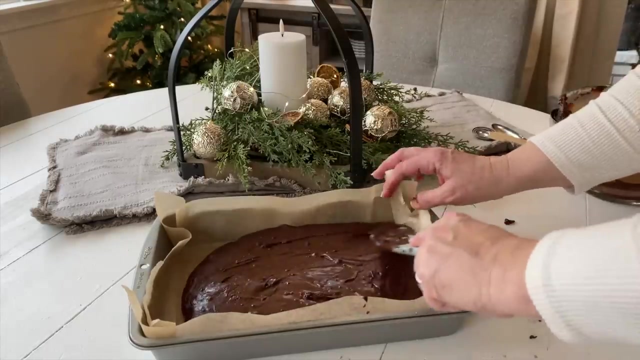 and then pour it in my prepared baking dish And, if you'd like, you could also stir in some chopped walnuts. And for a yummy, sweet and salty treat, you could stir in some chopped pretzels. So, and to make this fudge, I'm going to add a little bit of sugar. So I'm going to add a little bit of. 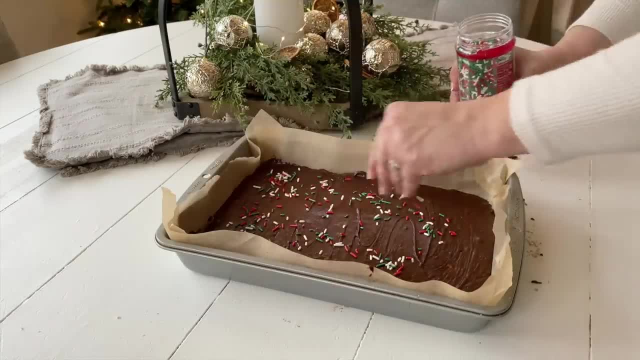 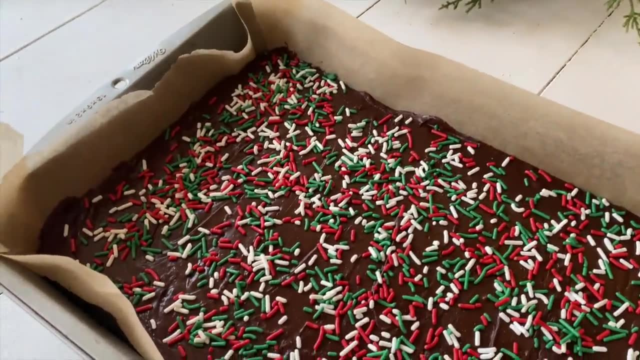 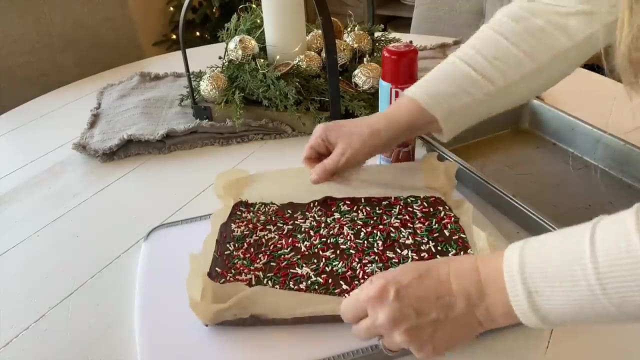 vanilla extract. And then, to make this fudge festive, I'm going to add sprinkles And then I'm going to pop it in the refrigerator to let the fudge set. Once the fudge is set, I'm going to cut it into pieces. I like to spray. 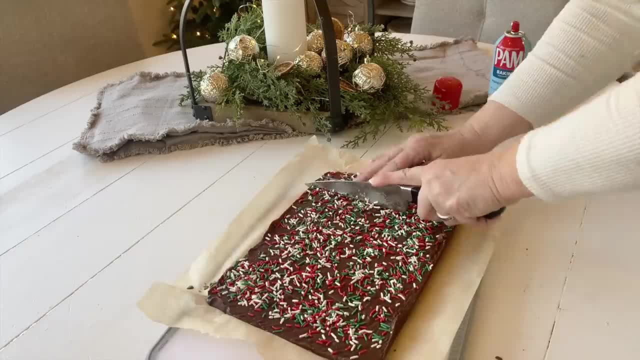 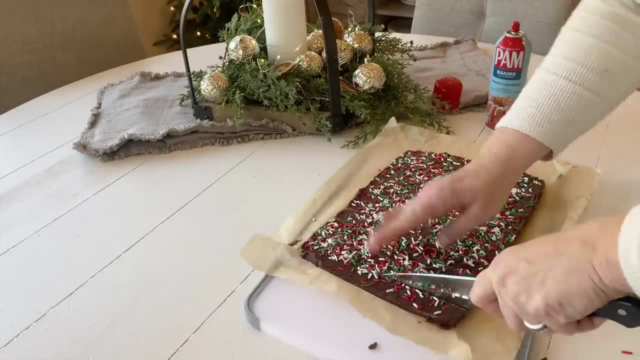 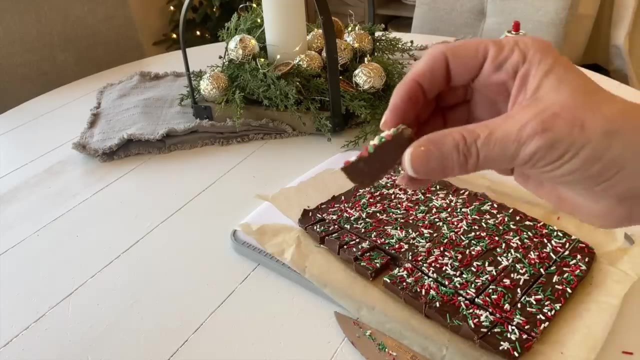 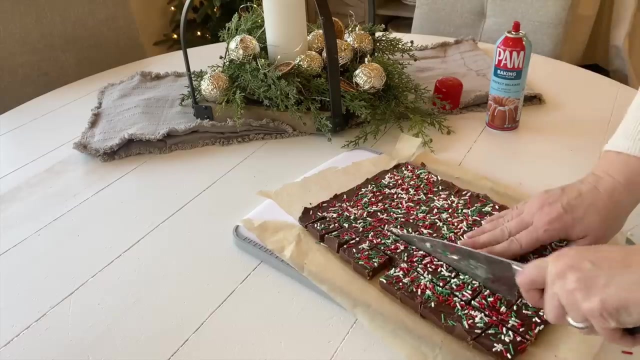 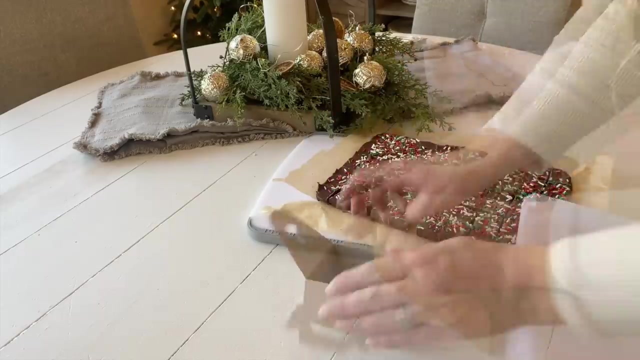 my knife first with some cooking spray and then it glides through the fudge. You can store this in an airtight container And if you want to gift this, there are so many cute seasonal gift boxes at the craft stores. I actually like these boxes. I get them at Hobby Lobby and I 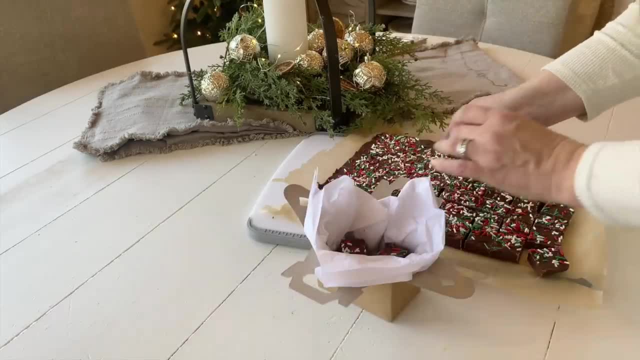 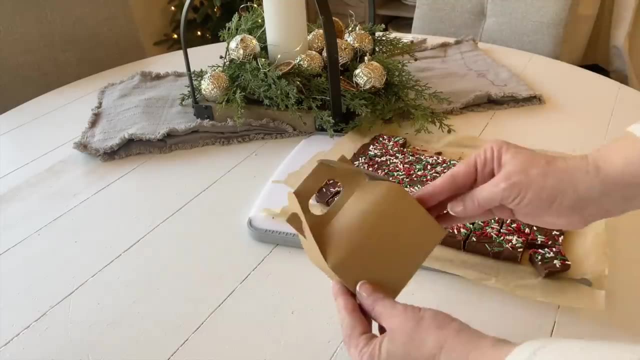 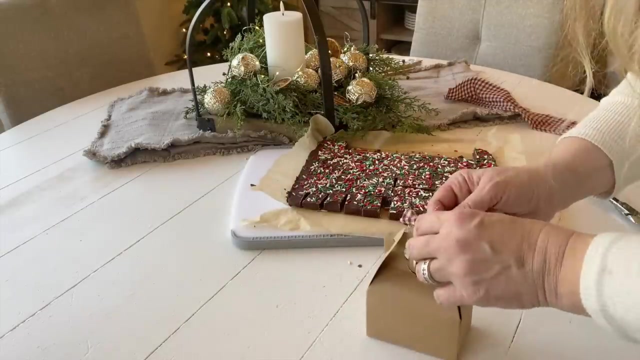 can use them year round. So I'm going to stick some tissue paper inside the box and add my fudge. And finally, I take a piece of torn homespun and add it to the top along with the bell, And this little gifty is done. These are great little favors to hand out if you're hosting a. 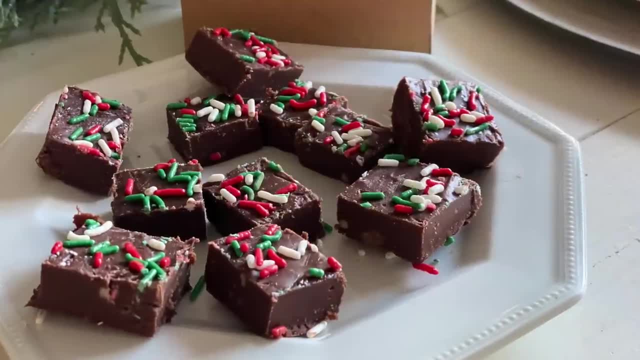 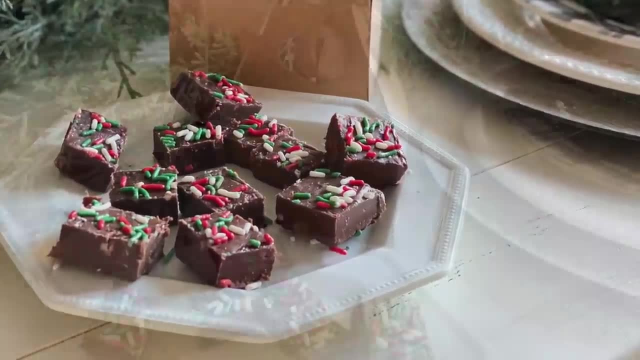 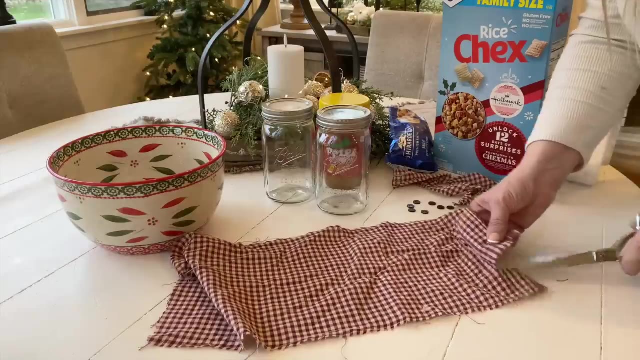 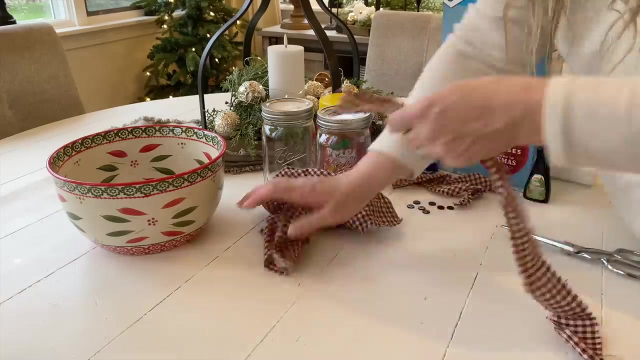 gathering, or to have it all over the place settings or to gift to friends and family. Next up, I'm going to make super cute Muddy Buddy snowman jars. I am using some torn homespun to make a scarf and then I'm going to hot glue some buttons on the jar. 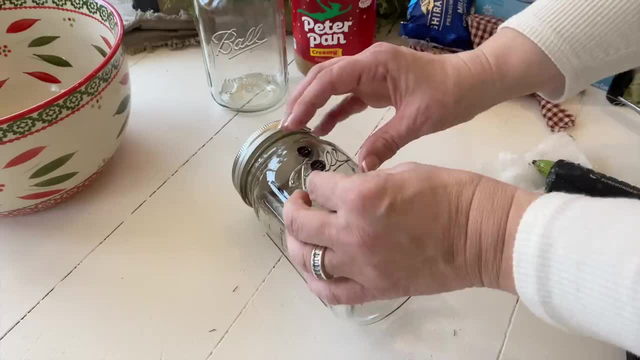 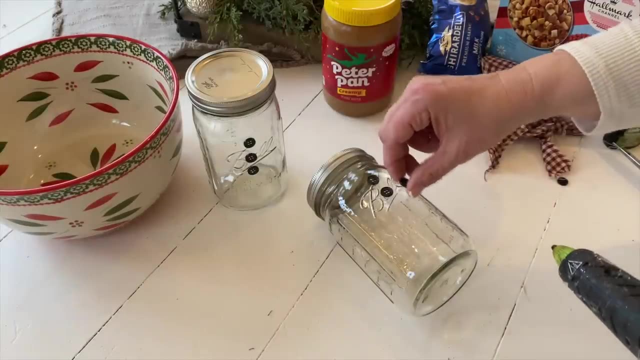 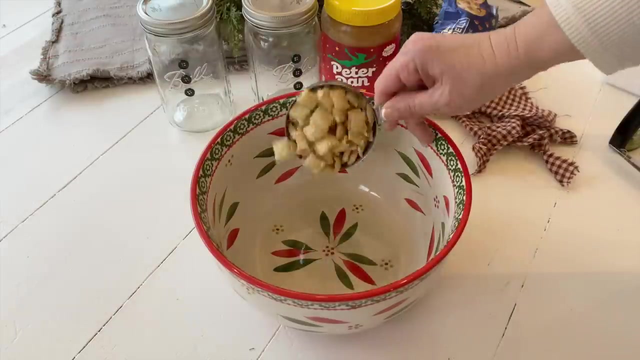 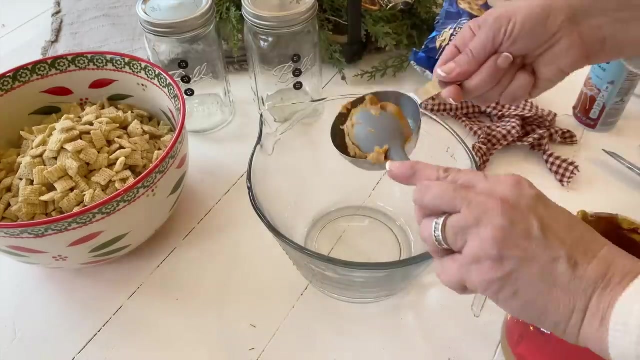 I'm using quart size mason jars, but you could use whatever size jar you'd like. Now I'm going to make the Muddy Buddies. In a large bowl I'm adding nine cups of rice check cereal, And in a microwave safe bowl I'm going to add a half a cup of peanut butter. 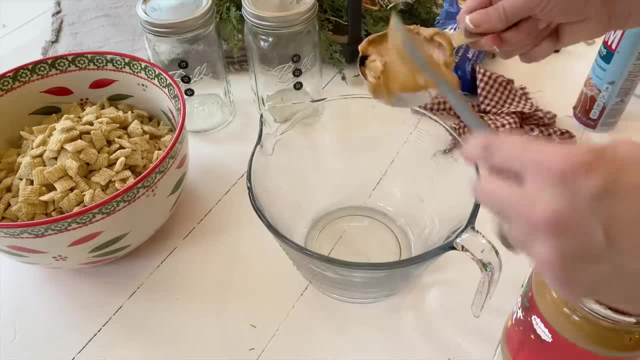 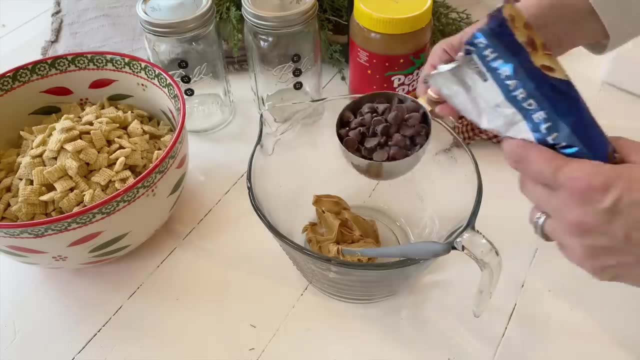 I like to spray my measuring cup with a little cooking spray, and then the peanut butter easily comes out, And then I'm adding one cup of chocolate chips and four tablespoons of unsalted butter, And I'm going to pop this in the microwave in 30 seconds. 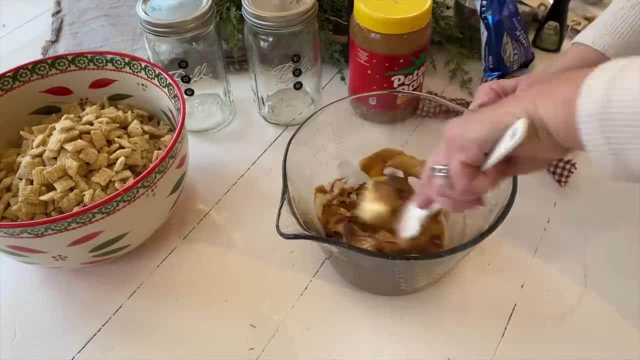 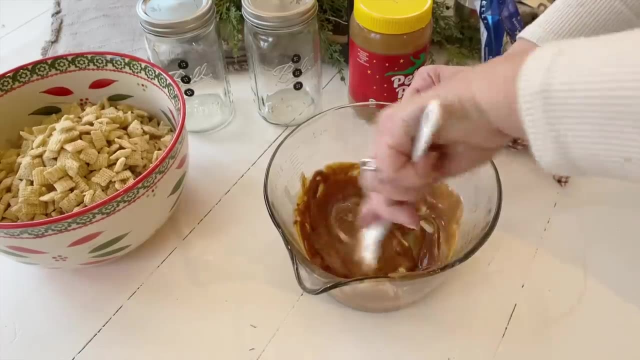 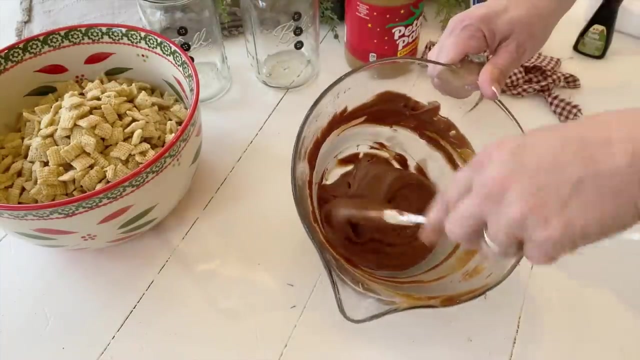 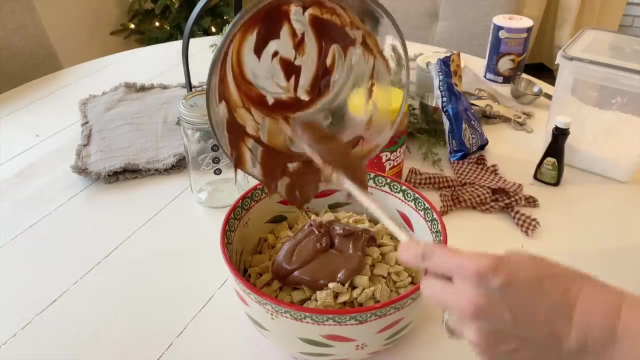 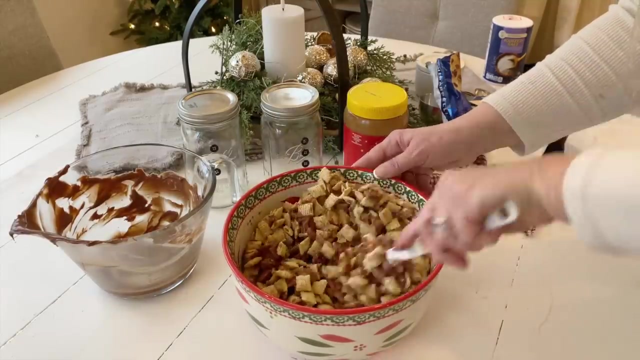 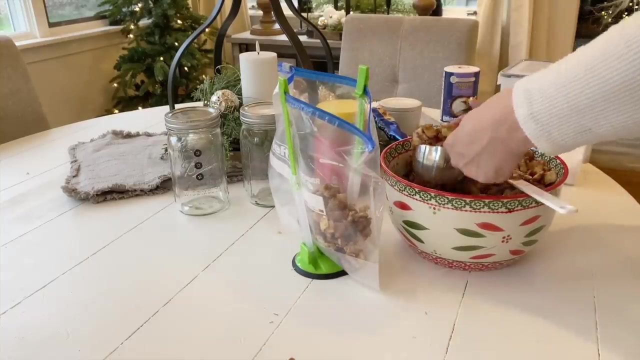 Increments until nice and creamy. Next I'm going to stir in pure vanilla extract and then pour the mixture over the cereal and gently toss to coat. Next I'm going to add three cups of the mixture to a gallon size storage bag And then I'm going to add two thirds cup of powdered sugar and give it a good shake. 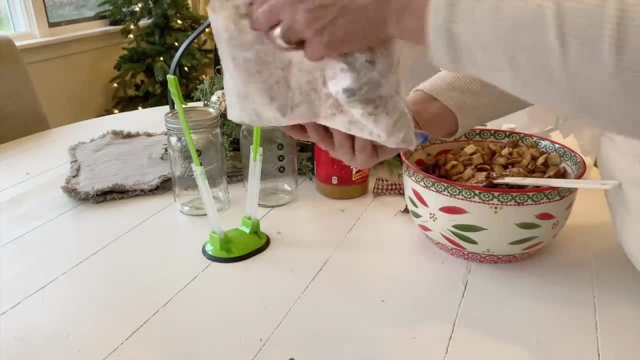 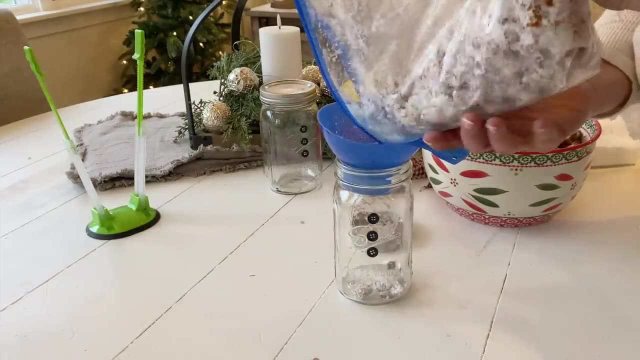 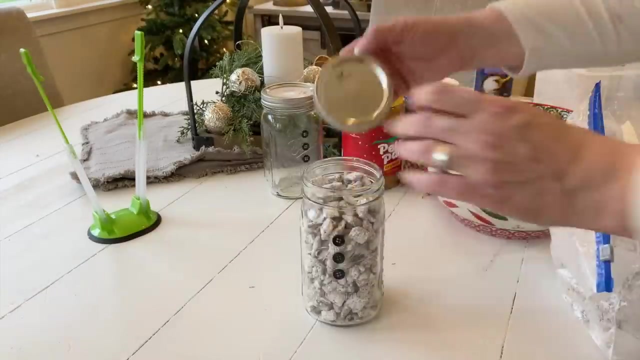 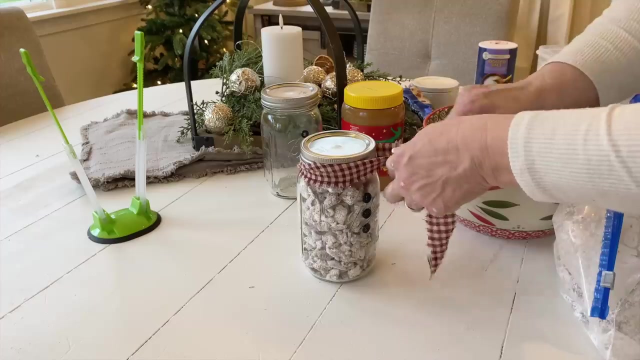 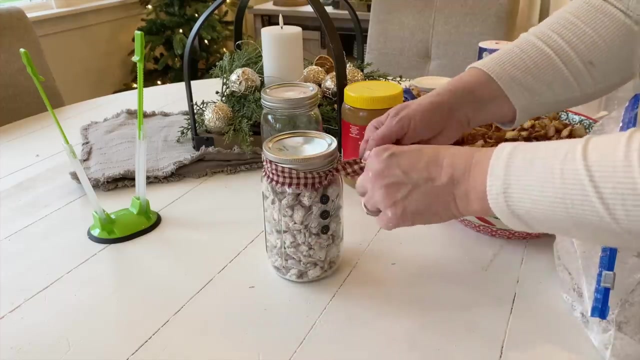 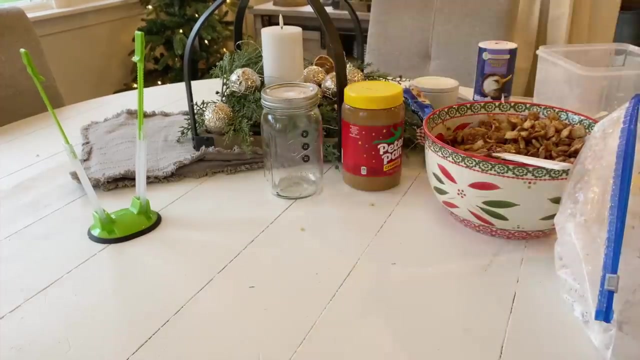 Next I'm going to add the Muddy Buddies to the jar, Then add the lid and then wrap around that piece of torn home-spun to make a scarf, and look what a cute gifty this makes. I continue working in batches with the. 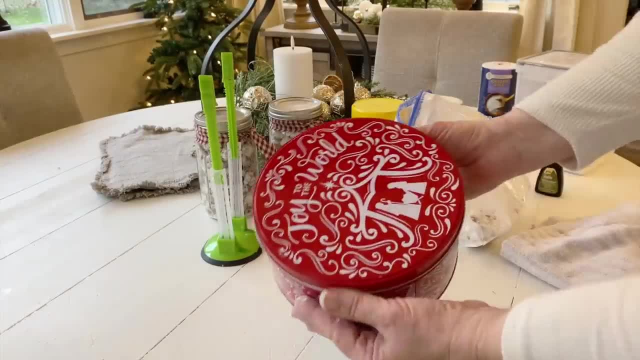 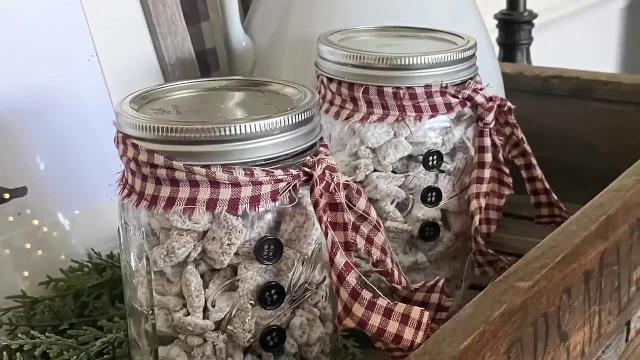 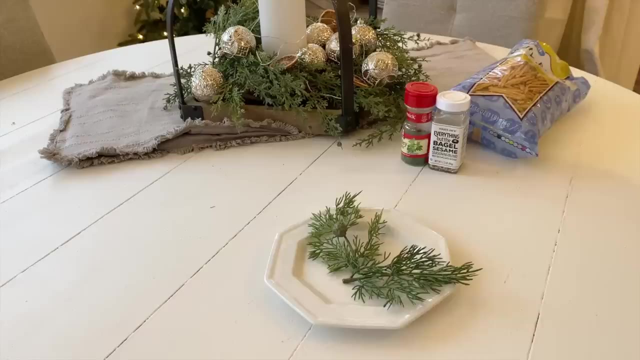 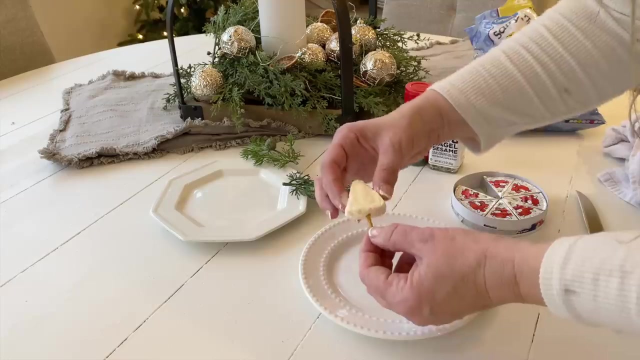 remaining muddy buddies and whatever I have left over I store in an airtight container. next I'm going to make cheese Christmas trees. I love making these for a fun appetizer, but they're also a really cute after-school snack for the kiddos as well. I add a pretzel stick. 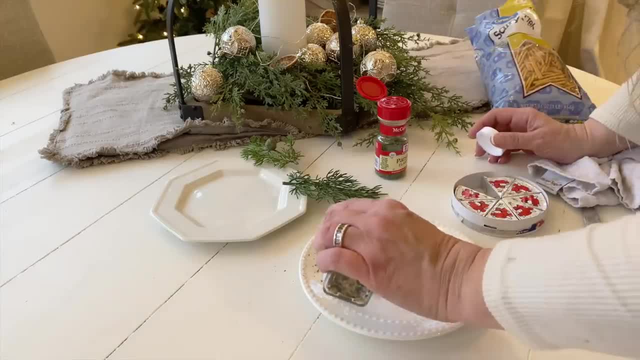 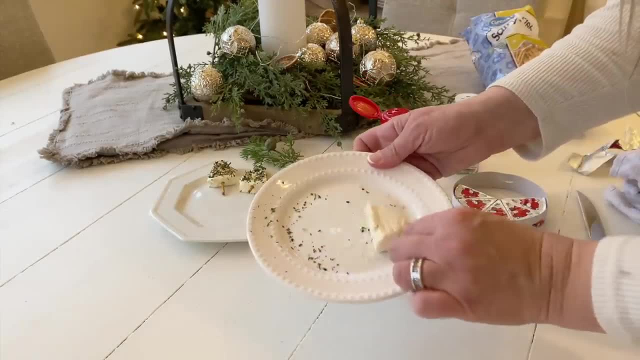 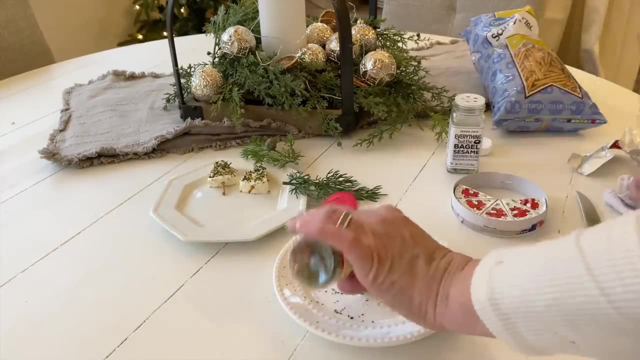 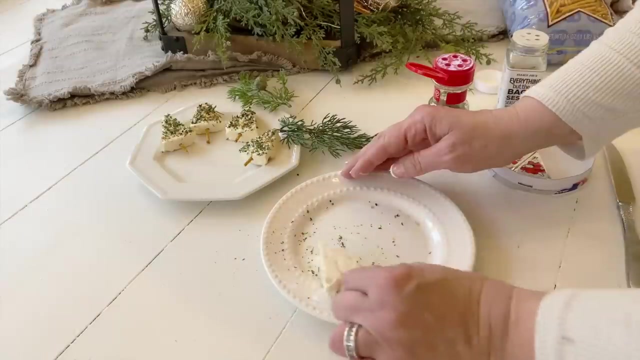 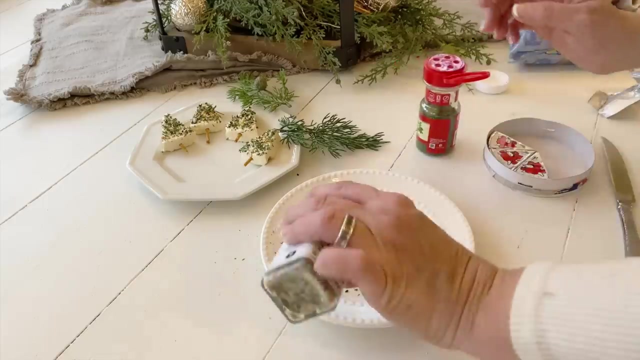 it's so easy too. you can make as many as you want for an appetizer, or just make a few for a little snack, and so I'm not wasting a lot of the seasoning. I go around and pat the cheese wedge on the plate with the seasoning and then I sprinkle any additional that I need to. 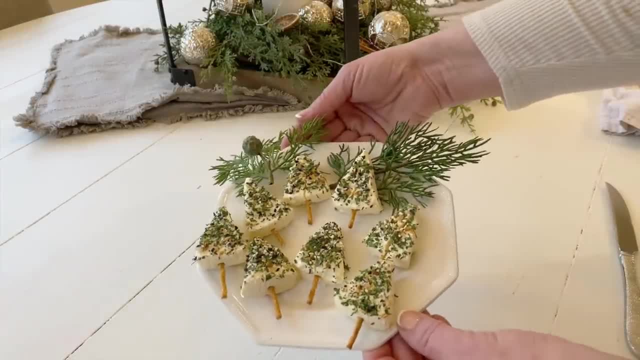 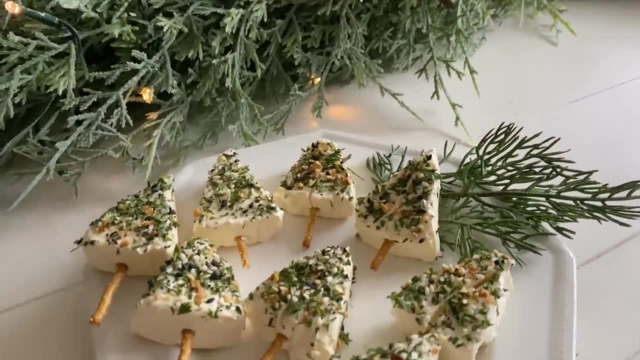 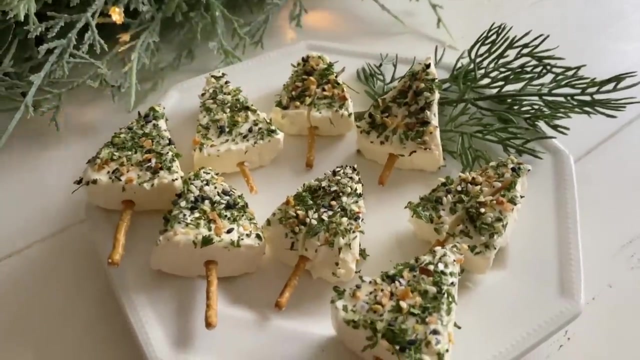 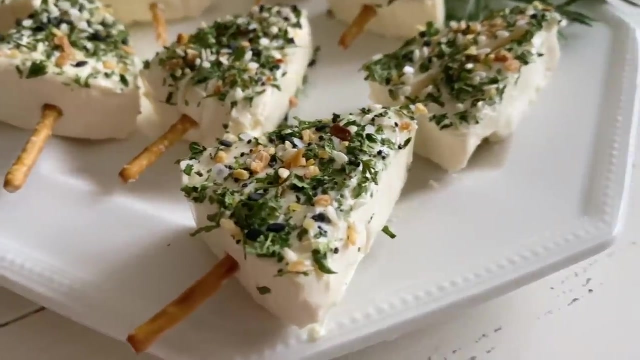 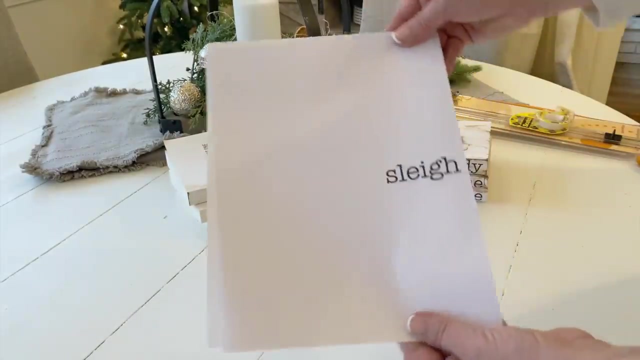 and look what a cute and festive appetizer this makes for any holiday gathering. next up, I'm going to show you how easy it is to make this Christmas book stack. I'm going to show you how to make this Christmas book stack using your local Toughly book shop in their book store. 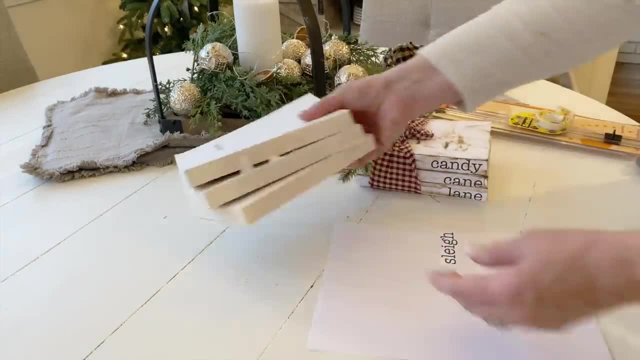 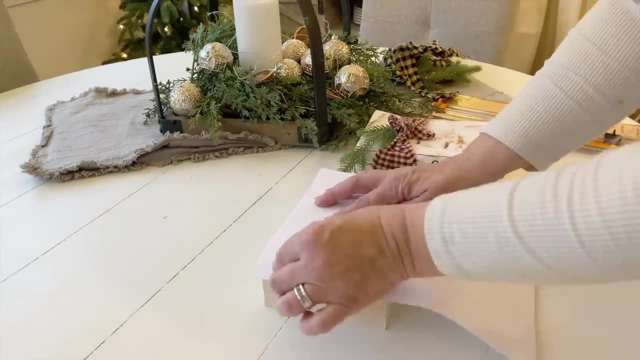 you can get it for free. on my blog there are over 20 different Christmas sayings to choose from. and then I'm using books from Dollar Tree. but shop your home or even the thrift store for some old books. first I'm going to trim the paper down, so I find the edge of my book and make a little crease. 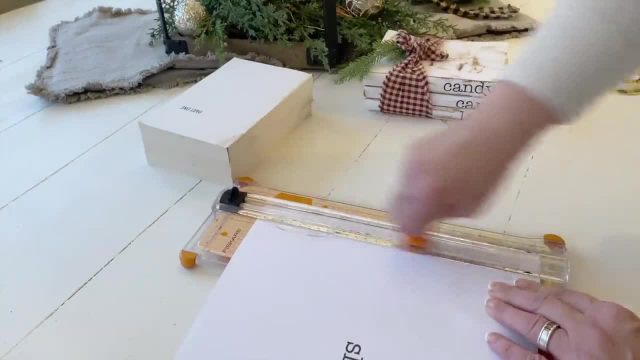 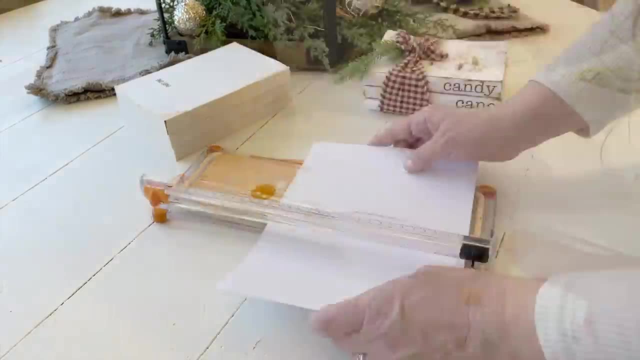 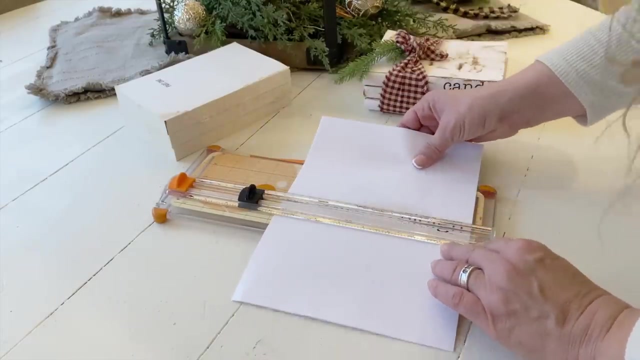 with my finger and then I'm going to trim that. there are score lines provided for the binding. if you could either do this by hand, but my little gadget here has a little score, so I'm just going to quickly score the paper. Also, I wanted to note I'm just using regular copy paper to make these. 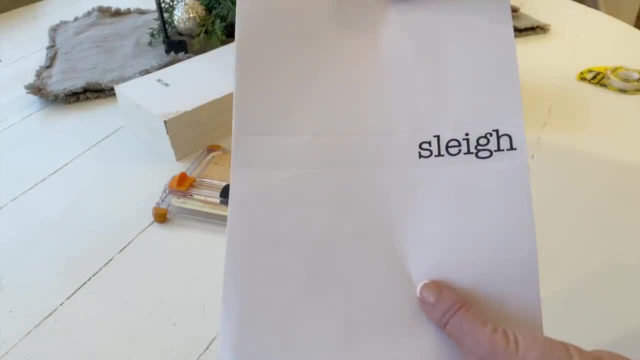 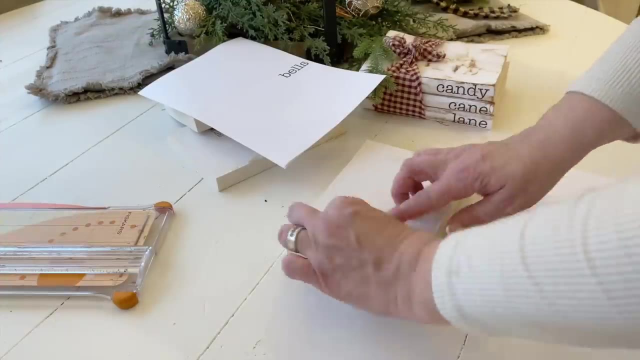 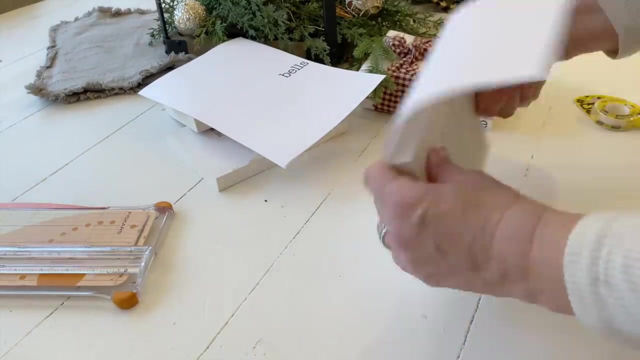 but you could use cardstock as well, And now I'm using some double-sided tape- or you could even use a glue stick, and I'm going to add that on top of the book and then wrap my book cover around it. and what's so great about this to you guys is that, after the holiday is over, I can easily remove. 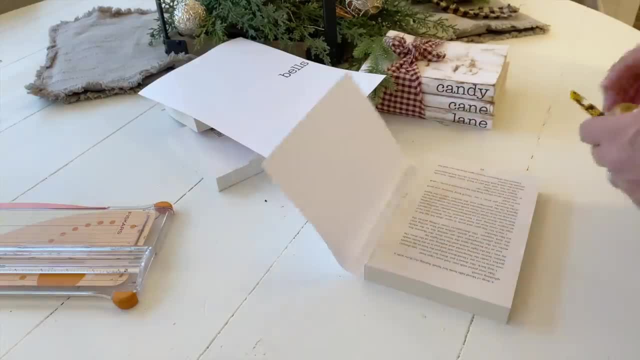 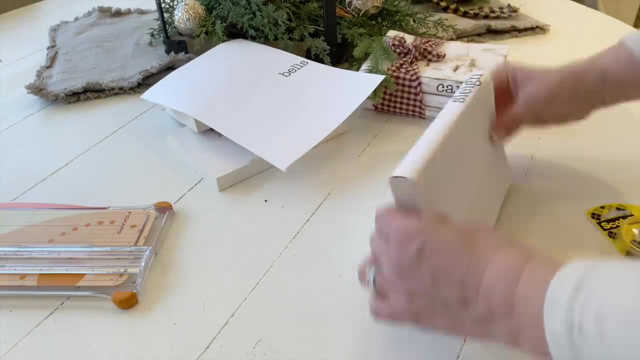 my book covers, if I'd like, and add new ones. I have several free book sack collections available on my blog and I'll include links for those in the description below. Also, I like to remove the book cover that the book comes with. It easily tears off. I've already done that on mine because I've 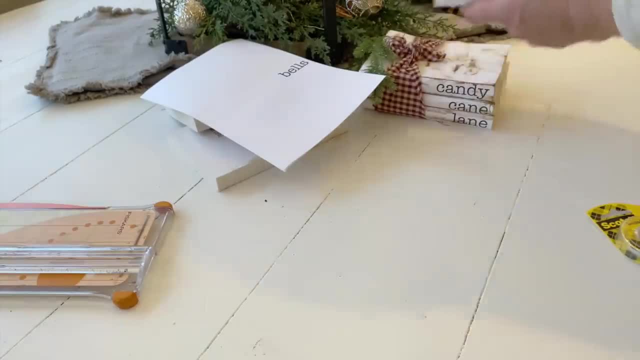 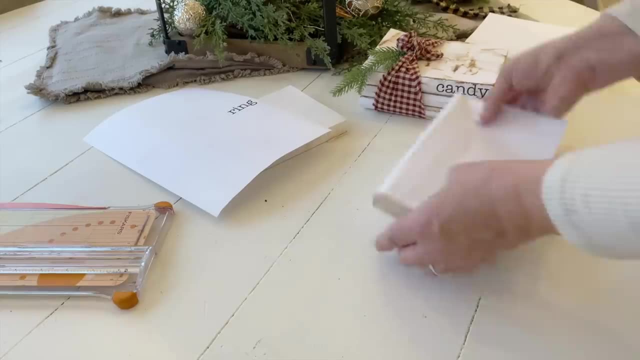 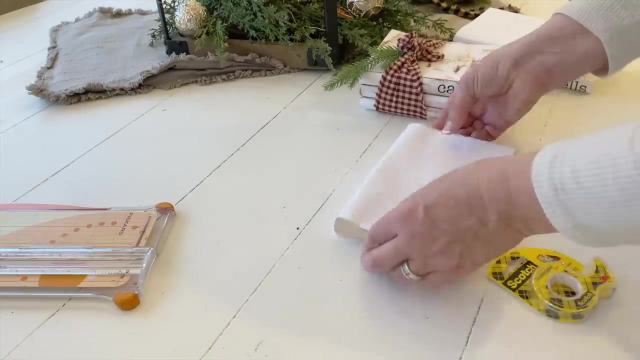 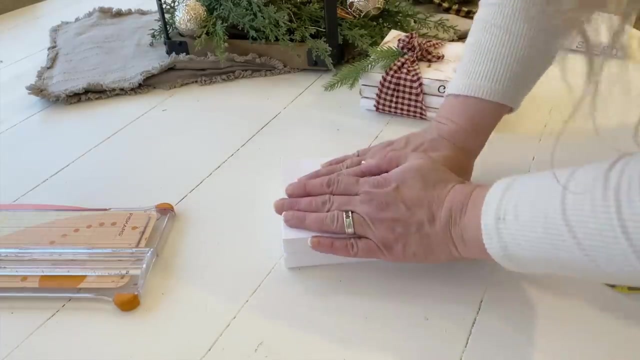 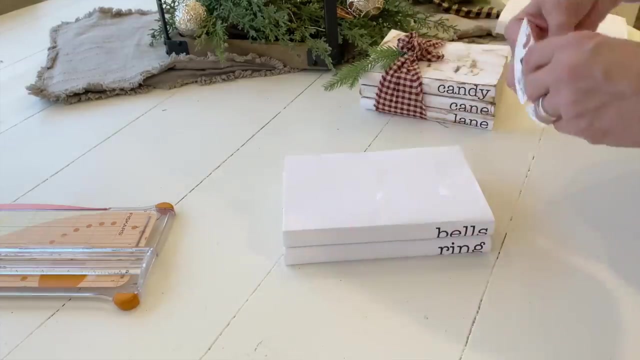 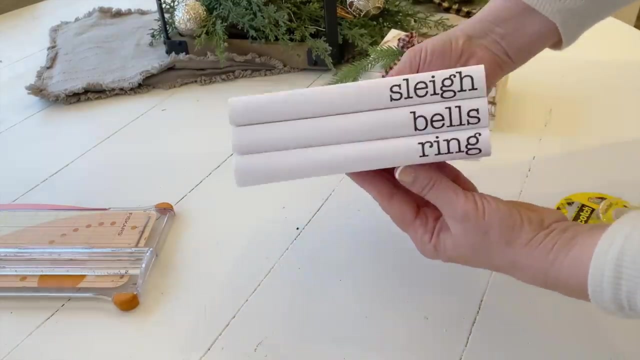 used these books for other book covers. Once I've added all my book covers, I'm going to stack them together and I'm using my double-sided tape to hold them together. You could use your glue stick as well, or, if you want a permanent hold, you could use hot glue, And this is how the book sack looks. I love it just like this, but if 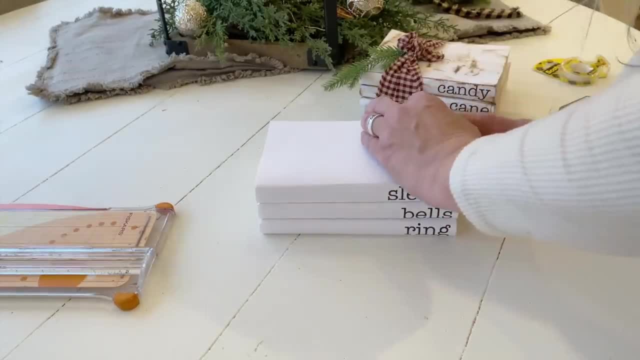 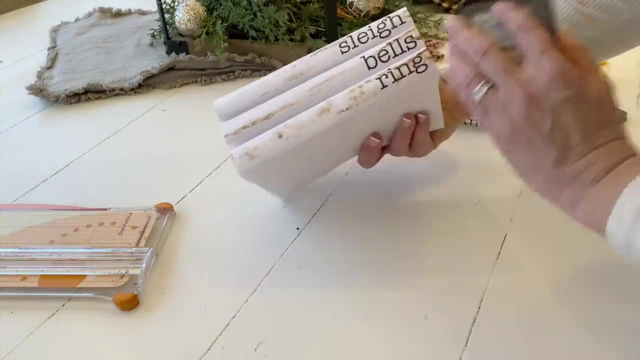 you want to add some distressing, I'm going to add a little bit of glue And then I'm going to add some distress oxide in the color vintage photo. I get it at Hobby Lobby. You can get it on Amazon as well. I'll include a link for that in the description below, And I'm gently rubbing it. 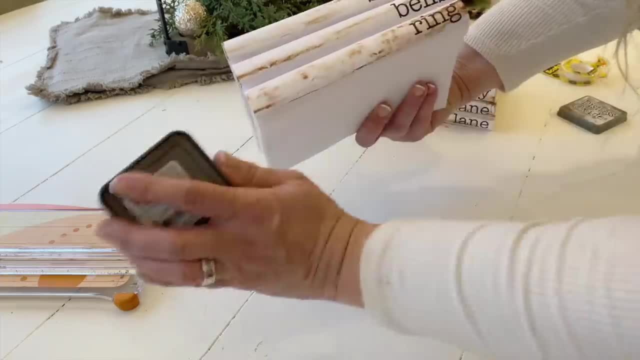 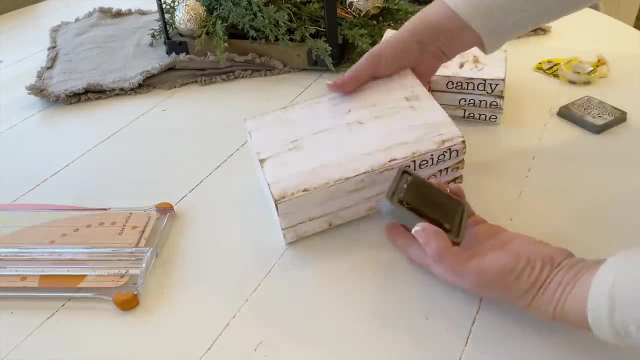 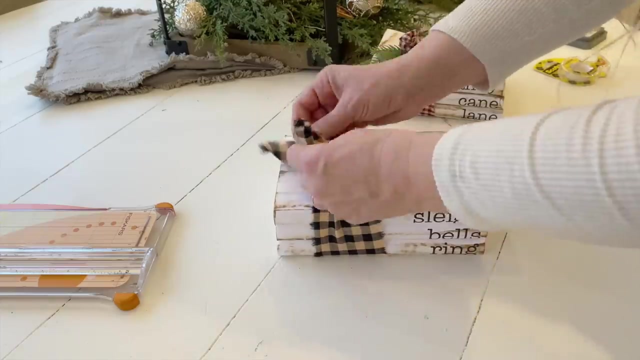 over the paper to give it a distressed look. And finally I'm wrapping the book sack with some torn homespun. I get my homespun at Hobby Lobby and I'm going to add a little bit of distress oxide to it. And then I'm going to add a little bit of 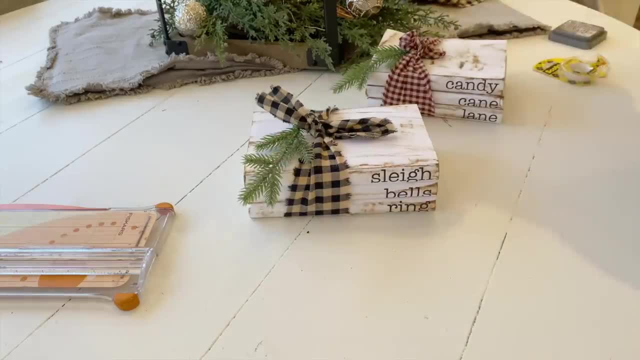 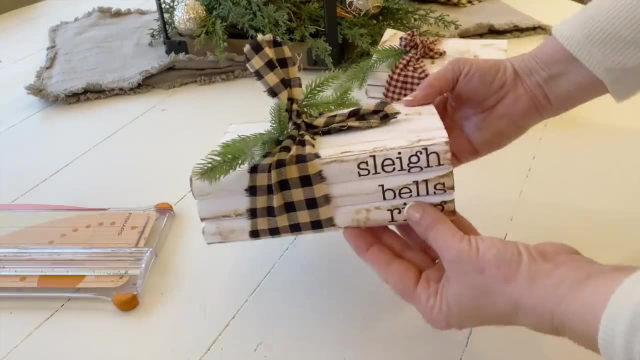 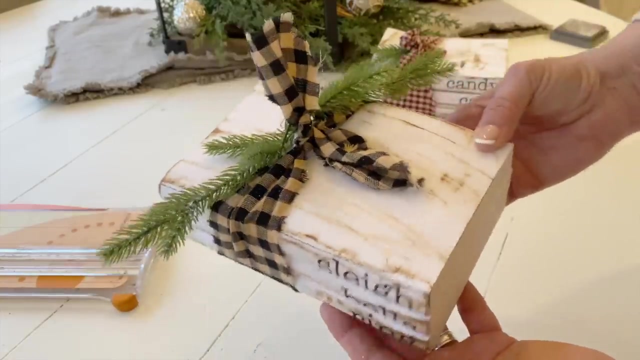 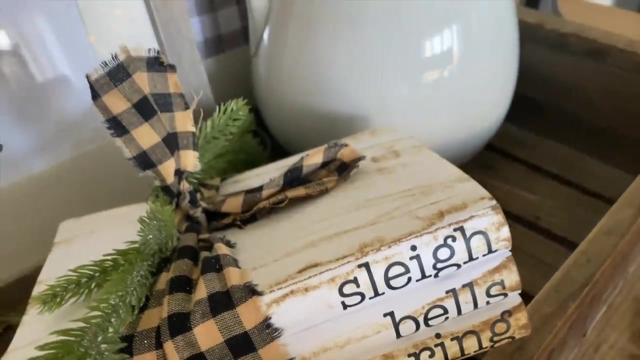 green picks as well, And look how darling this book stack turned out, and so easy to make too. You could use this for decor in your home or to even make as a gift. Next up, I'm going to share another fudge recipe. This is peanut butter fudge. I'm going to add a little bit of green picks as well, And I'm going to 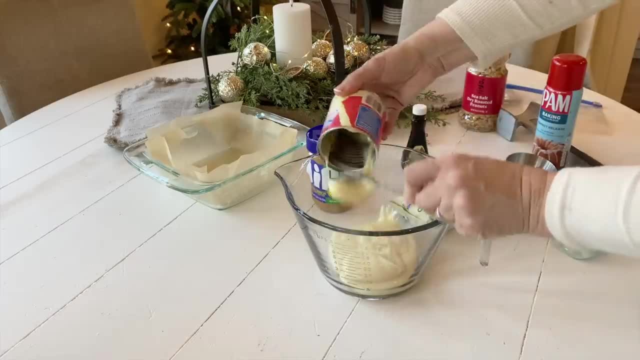 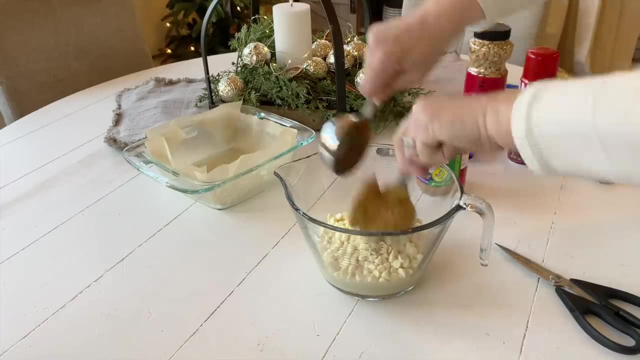 add a little bit of green picks as well. And I'm going to add a little bit of green picks as well- Super easy to make- To a microwave safe bowl. I'm going to add a can of sweetened condensed milk. I'm also going to add an 11 ounce bag of good quality white chocolate chips, If you cannot. 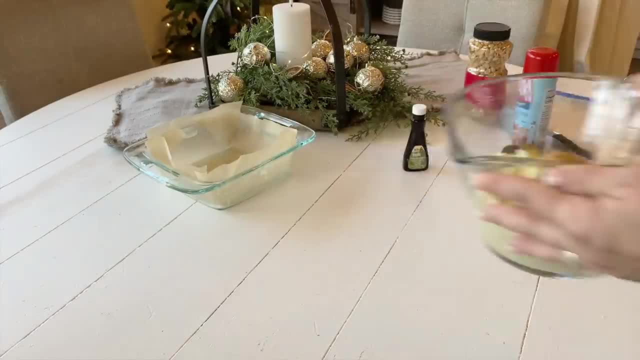 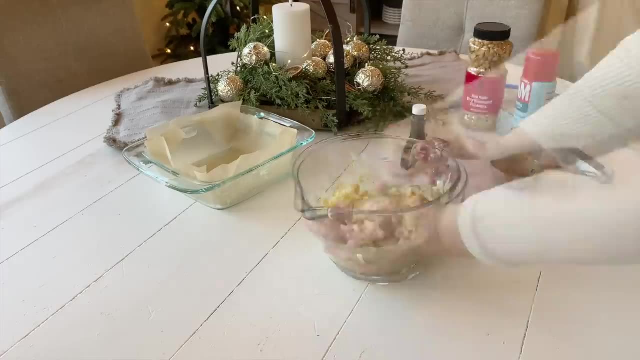 find the 11 ounce bags, just add two cups of white chocolate chips along with a half a cup of crunchy peanut butter. You can use creamy too, but let me tell you the crunchy is really, really good. And then I'm going to microwave this in 30 second increments until it is creamy. 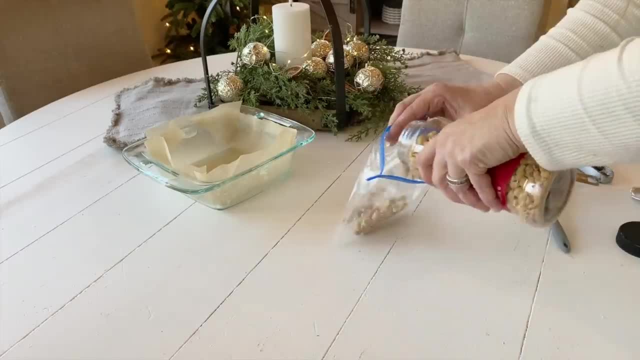 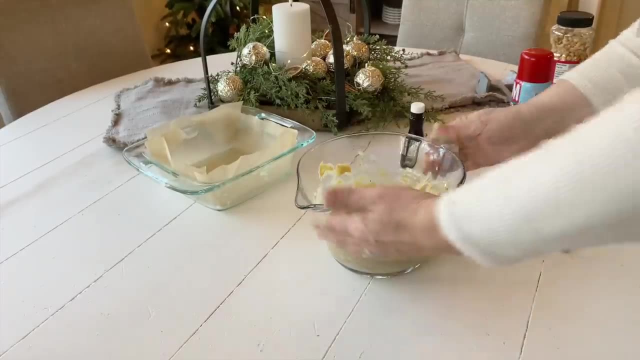 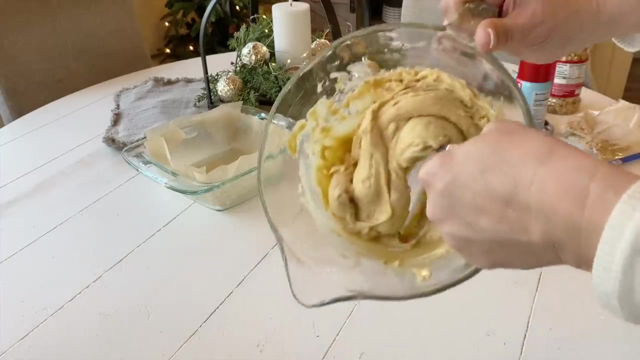 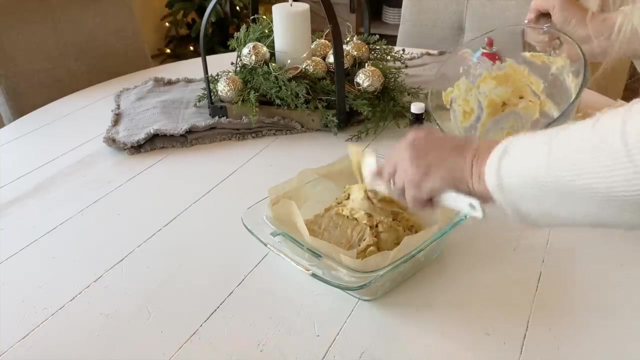 Meanwhile, I'm going to crush up about a half a cup of peanuts to sprinkle on top of the fudge, And once the mixture is nice and creamy, I'm going to stir in some vanilla extract, And then I'm going to pour the mixture in a baking dish that I lined with parchment paper. 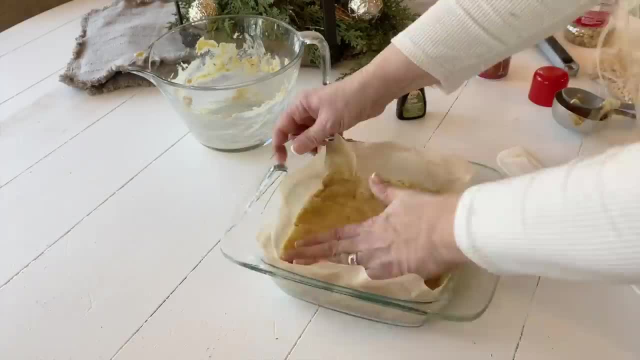 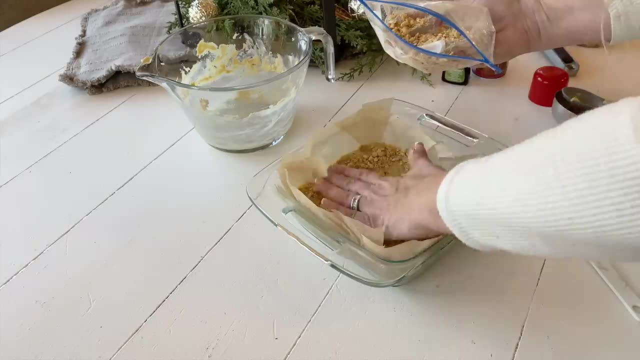 and spread it evenly. You could use the spatula also. the hands work really well For this one too. Next, I'm going to sprinkle the top of the fudge with my crushed peanuts. I also like to sprinkle on some sea salt as well. It is so yummy. And then I'm going to place this: 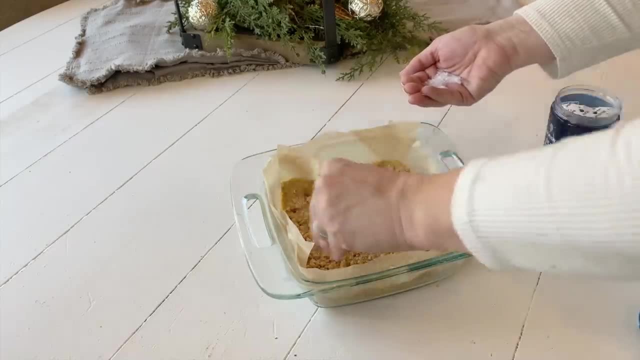 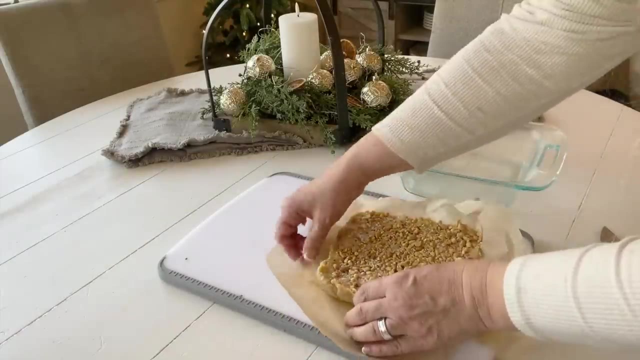 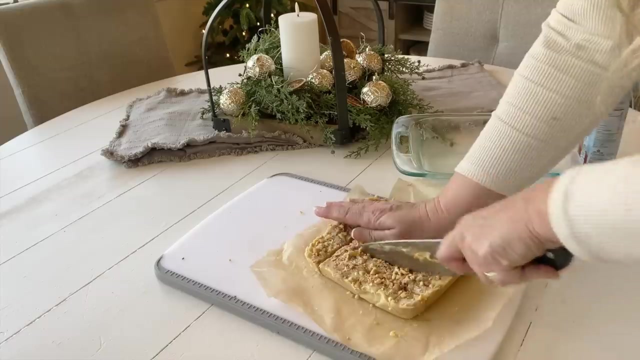 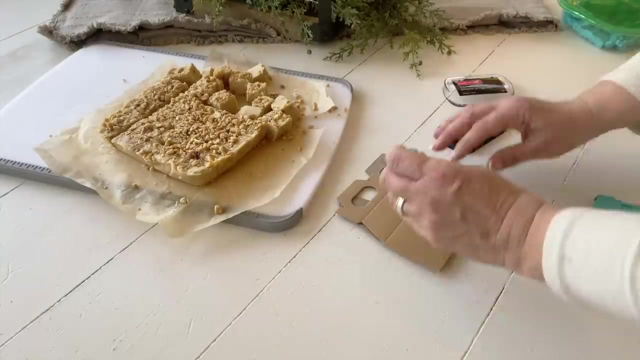 in the refrigerator to set. Once the fudge is set, I'm going to cut it into pieces, like I did with the chocolate fudge. I like to spray my knife with some cooking spray so I can easily cut through the fudge. And to give this, I'm using one of these boxes from Hobby Lobby And I'm going to stamp this. 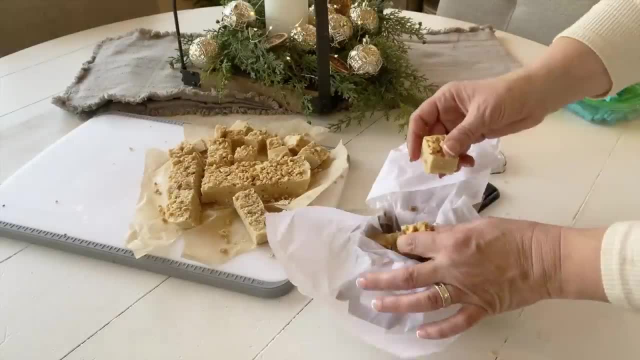 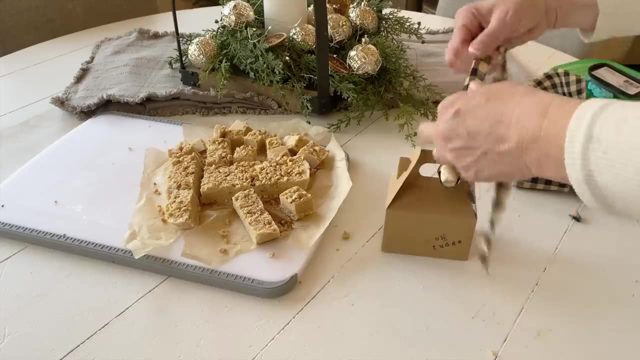 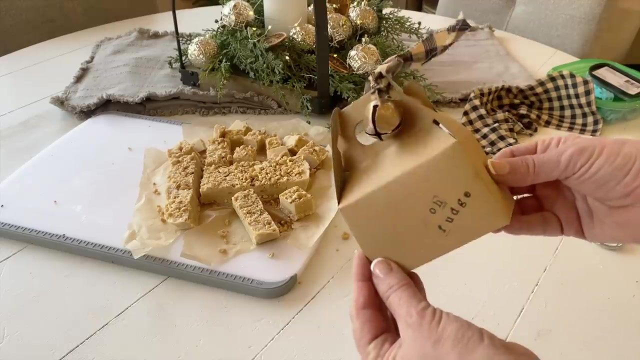 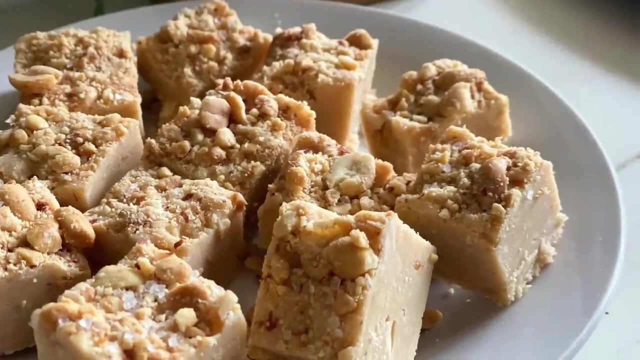 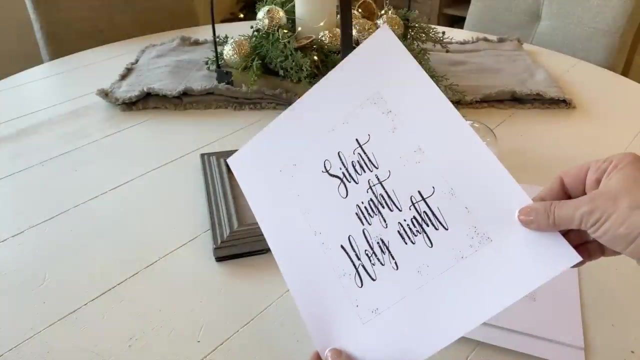 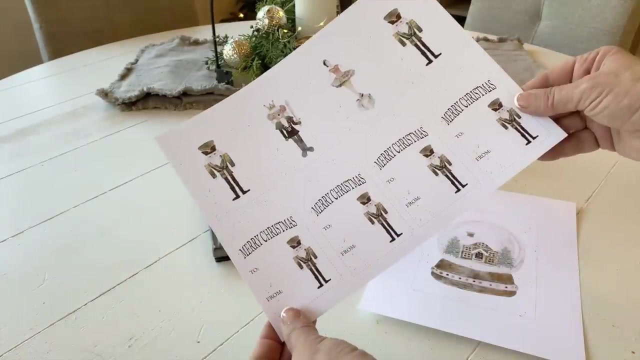 saying, Oh, Fudge, which is from one of my favorite Christmas movies, A Christmas Story. And then I add some tissue along with the fudge And place this side of it in the perfect place to cover it. The fudge is ready. For this one, I'm using an E privet bag. The bag must be tight so I can wear it like a. 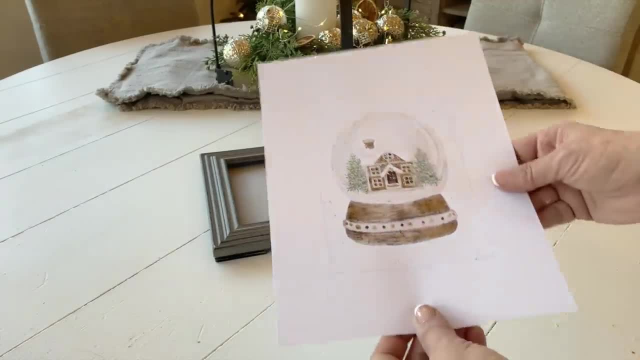 t-shirt or go anywhere without bringing ed substaci Once the fudge is all under the spiders in the bag. ihn parents are going to stay in the house пять for hours a day because when they buy Christmas ceviche they are going to need. 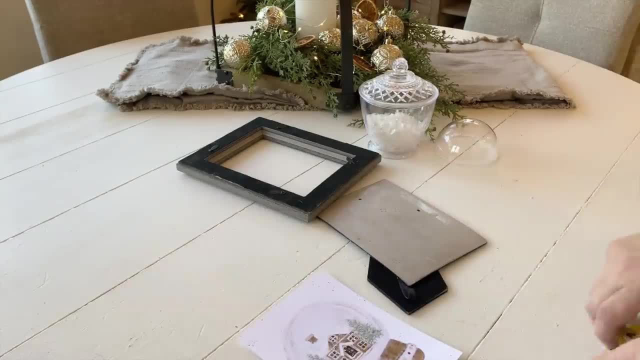 to behave нужen to them. They only make Boxes and these still don't last too long. Some of these do, some don't, some don't even happen to me on cardstock, and then i'm going to cut it down to a five by seven. this comes in a five by seven and 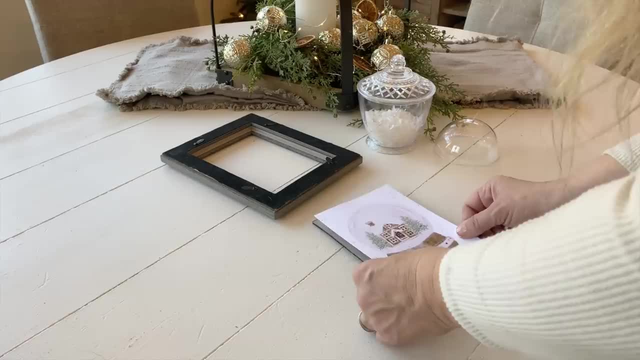 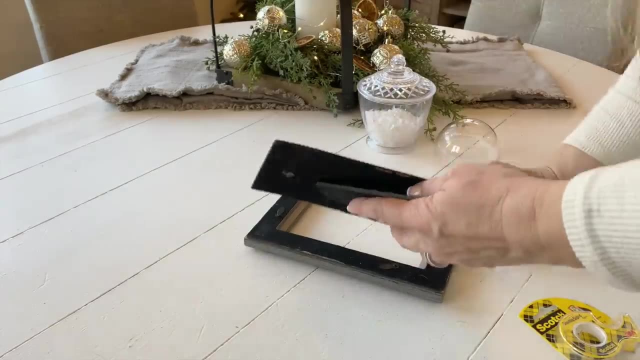 an eight by ten, and then i'm going to frame this. i just added some double-sided tape to this frame that i had on hand. you can find frames anywhere- the craft store, thrift store, dollar, tree, home goods, you name it- and then i'm going to add it, without the glass, into the frame. 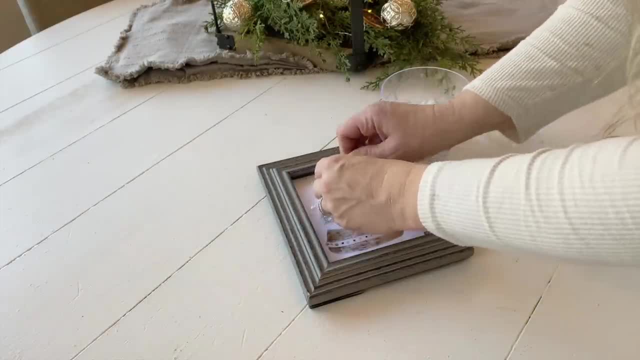 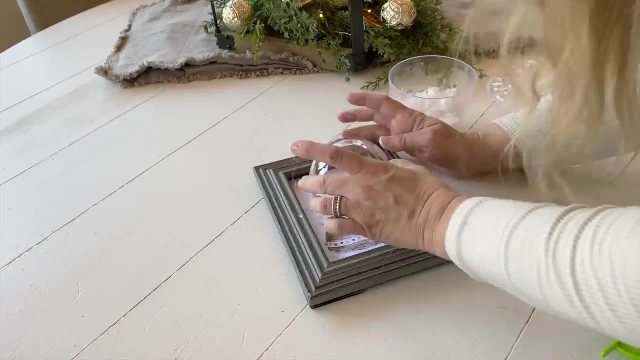 next, i'm taking this fake snow that you can get a dollar tree or the craft store and i'm going to place it on top of the snow globe pitcher. and then i have this clear ornament. it's like a half clear sphere ornament. you can find them year round, even at hobby lobby. they're. 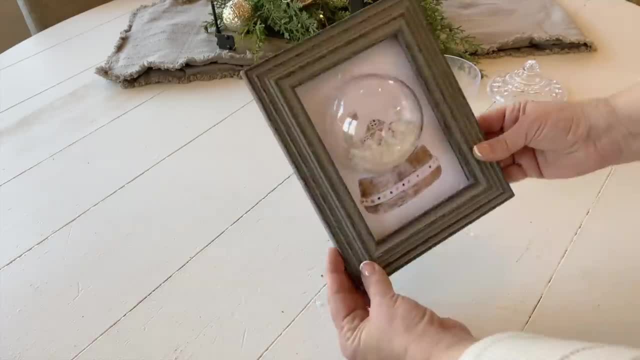 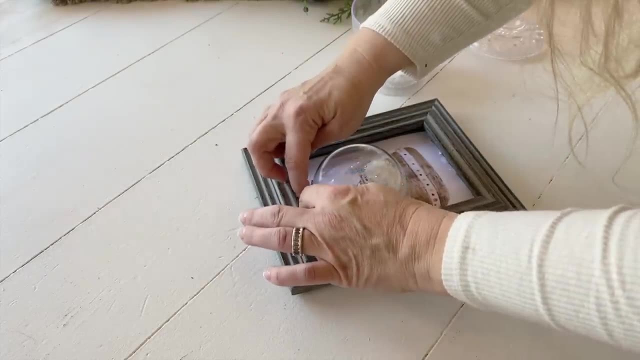 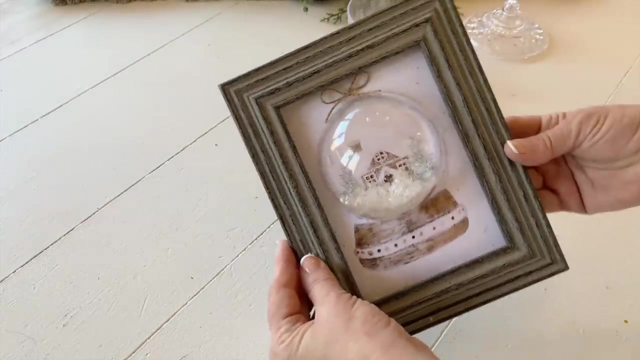 usually, like in the glass section, i'm going to add some hot glue around the rim and place it on top of the snow globe pitcher. and finally, to cover the top, i made a cute little twine bow and i'm going to hot glue that to the top and look how cute this turned out- and so easy to make too. 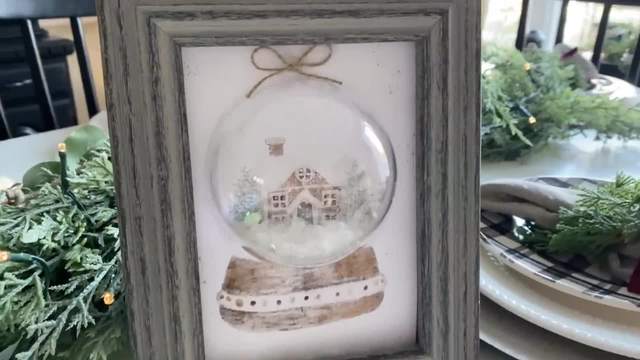 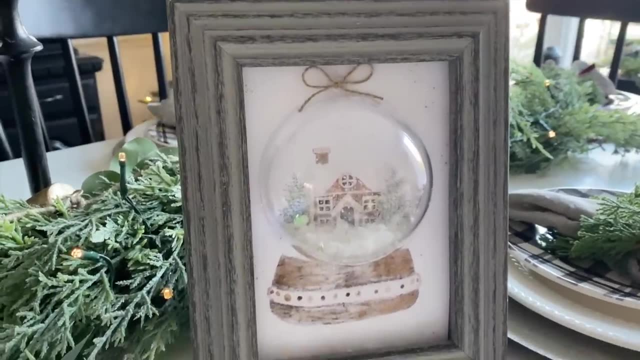 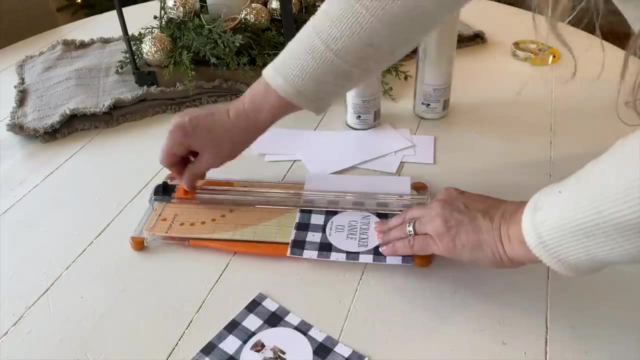 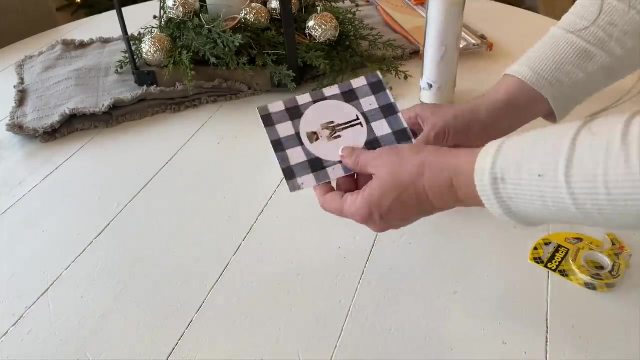 so next up also in the free printable collection are these candle wraps, and this is so easy to do. so you'll need these filler candles from dollar tree, and then i reuse these every season. so i just tear off the previous season candle wraps and add the new ones. you can use double-sided tape. 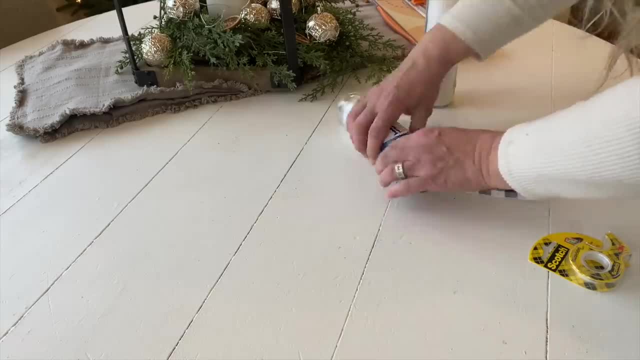 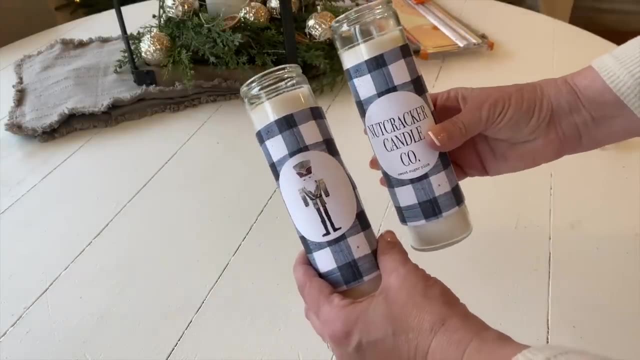 like i am here, or you can even use a glue stick. i simply cut out the candle wrap and then i add it to this pillar candle. and sometimes i wrap the pillar candles with some twine or add a little bow, but i love these candles just like this. and look at how.